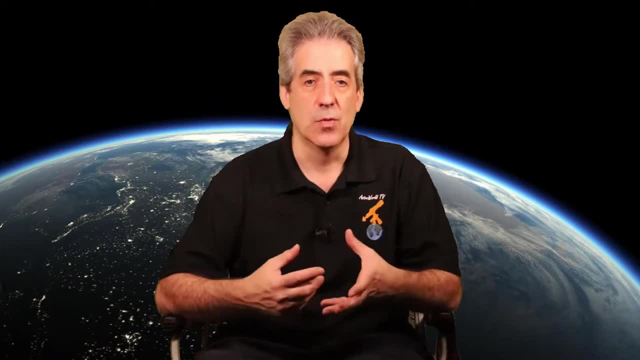 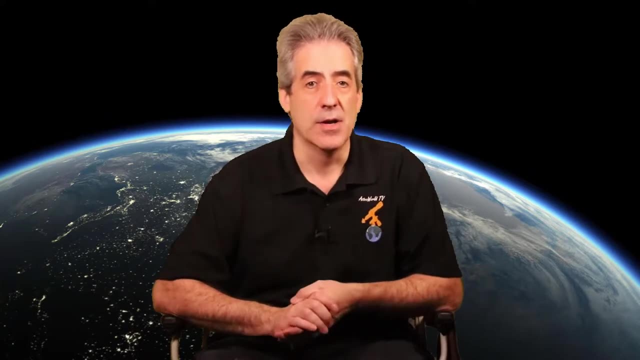 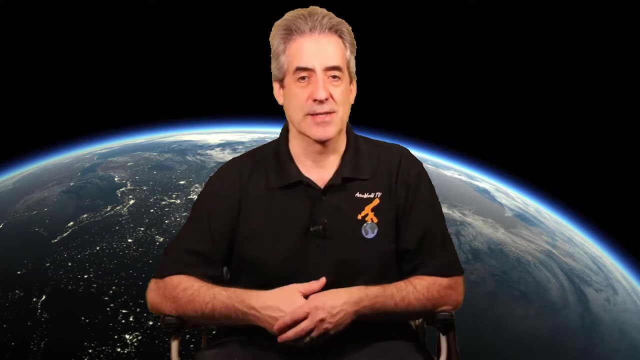 please subscribe and hit the bell so you can get all the notifications when Astroworld posts new data. And don't forget to visit astroworldwebcom, our new website, in order to check out all the players at Astroworld. That being said, let's start taking a look at refracting telescopes. 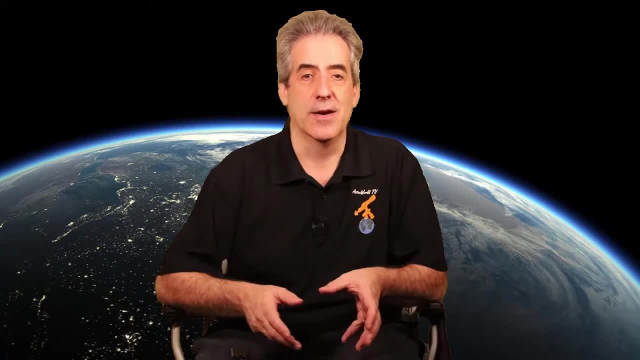 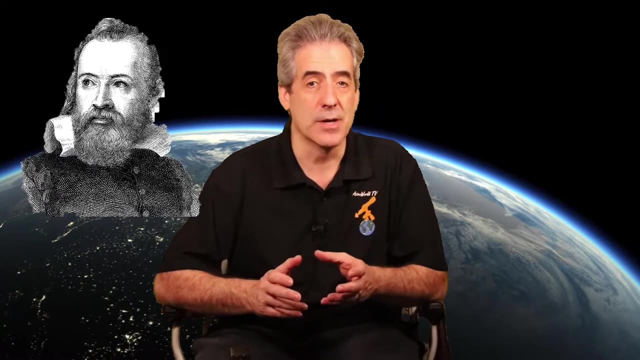 The refracting telescope is the oldest type of telescope out there and, even though Galileo made the telescope extremely popular by being the first recorded person to point the telescope skyward, it was originally used militarily and thought to be invented by Hans Lippershey in. 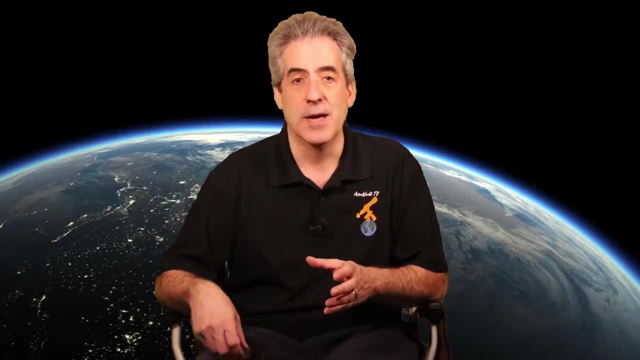 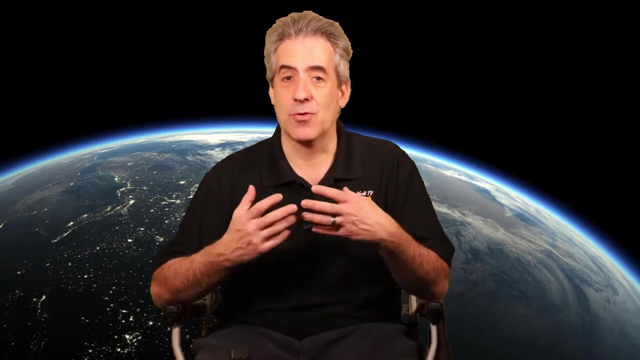 Denmark in 1608.. It was a small telescope and had a magnifying power of three times the power of your eye. Galileo, after hearing about this invention from a colleague, was inspired to build his own telescope. without seeing Lippershey's invention, believe it or not, He went on to make great 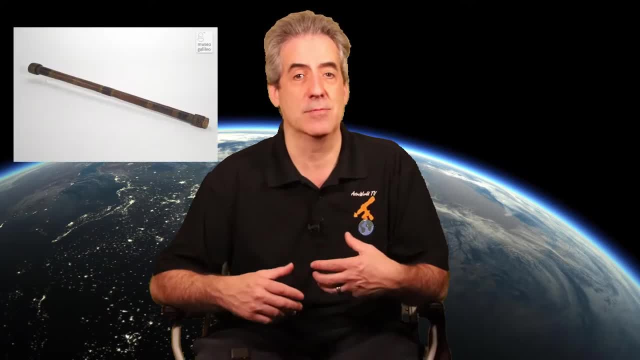 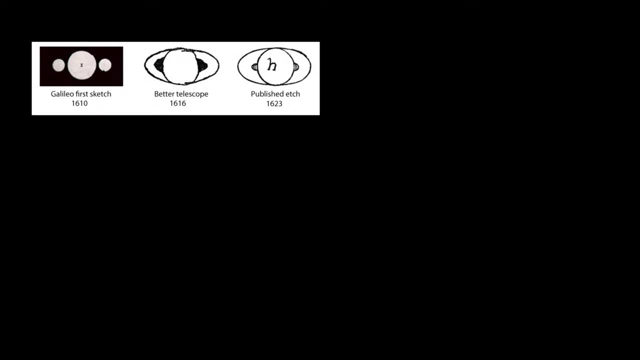 improvements and eventually he built a telescope that would get approximately 20 times the power of your eye and enable him to discover the rings of Saturn sunspots, four of Jupiter's moons, as well as a glimpse of diffuse light arching across the sky, which would later be known as. 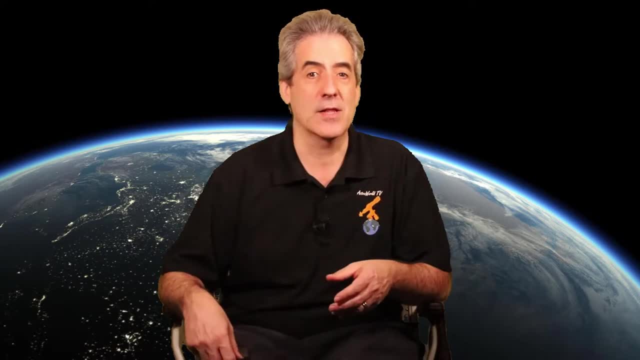 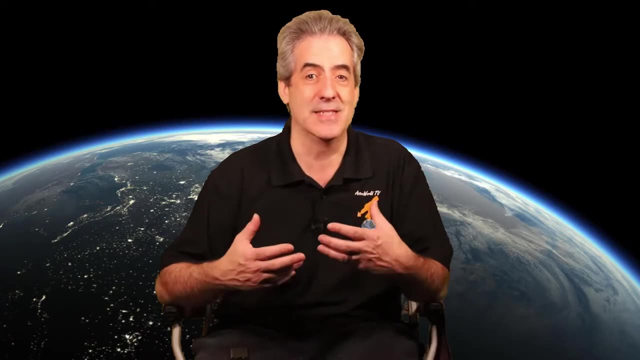 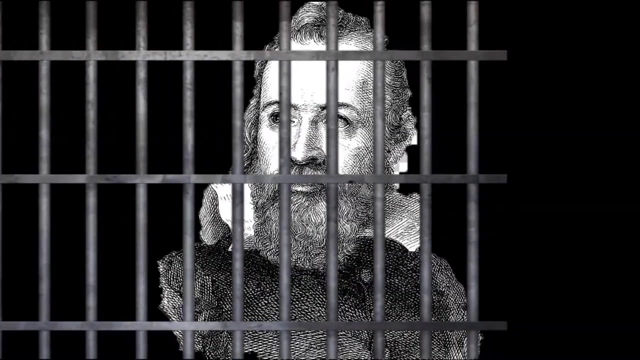 the Milky Way Galaxy, Galileo would quickly become convinced that Copernicus' heliocentric model was absolutely correct, a position that would ultimately see him put under house arrest by the Catholic Inquisition until his death in 1642.. He was actually in jail for nine years because of this theory. 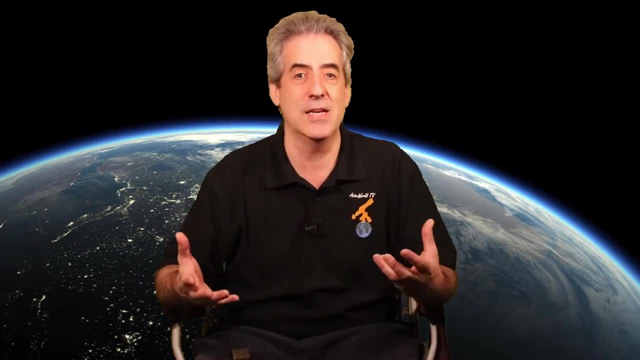 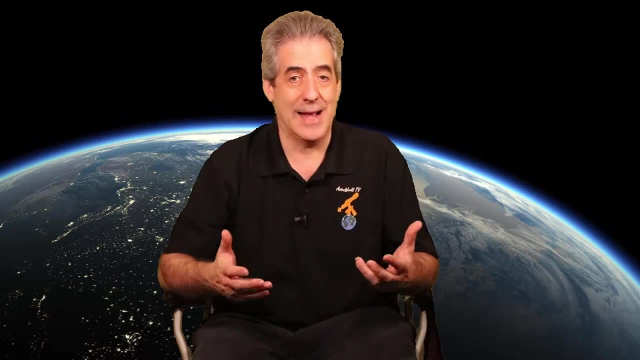 Now, that's just some of the history of the refracting telescope. Now let's see what it can actually do for us. A refractor is built with glass lenses and a tube and an eyepiece. It can be built with numerous elements based on the design. 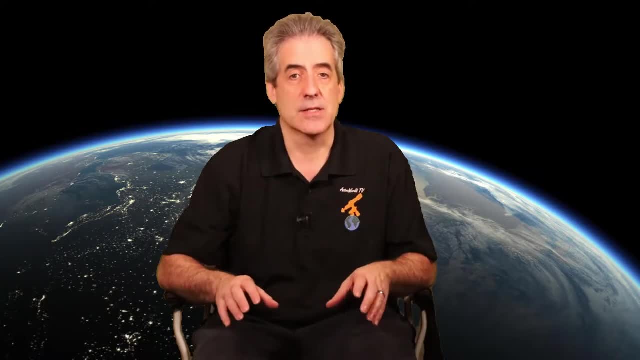 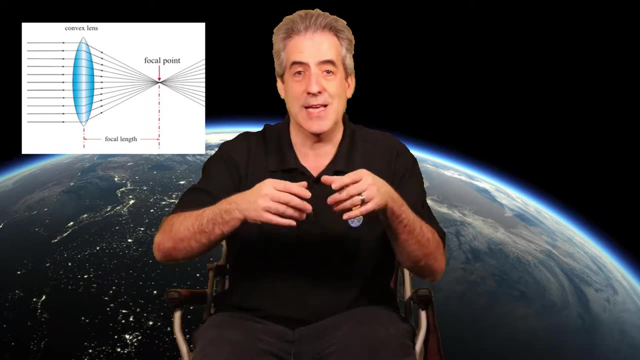 but the basic concept of it is this: The lens is a convex lens, which is a lens that is actually curved on both sides so it can focus an image at the focal point, which is actually somewhere in the tube. The eyepiece then takes over and then magnifies the actual image in order to make an 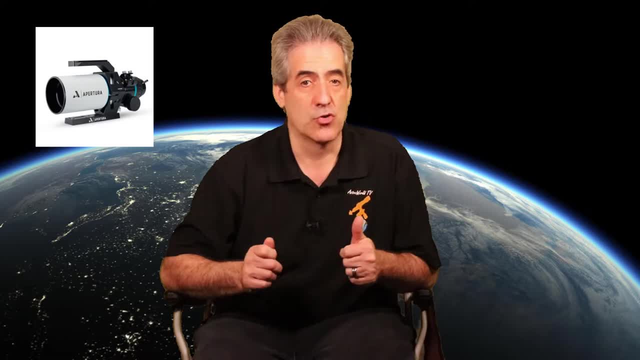 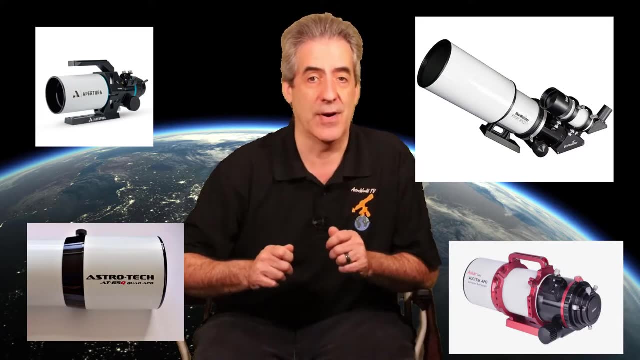 image that you can view. You can have a doublet, a triplet, a quadruplet or a quintuplet refractor and this name is called a refractor. This name signifies the amounts of elements in the refractor. All of them have an individual purpose. 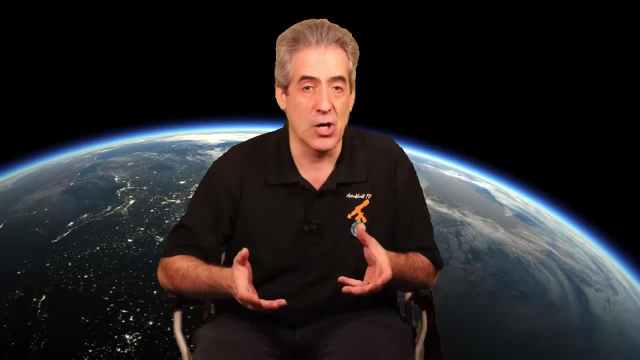 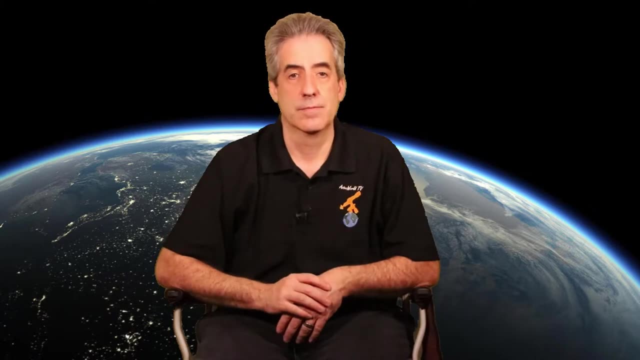 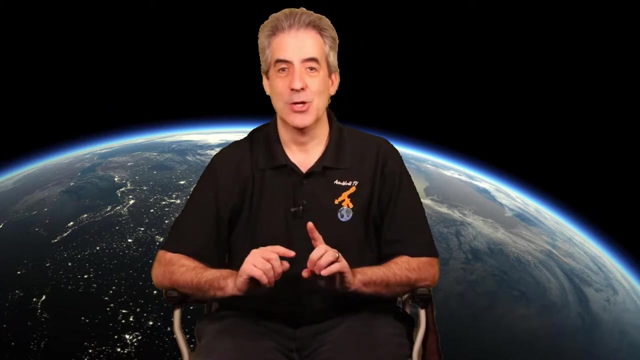 which will be discussed in my next video. So, when it comes to astrophotography, what are the pros and cons of a refractor? So let's start with the pros, First of all. no collimation needed usually, Usually. 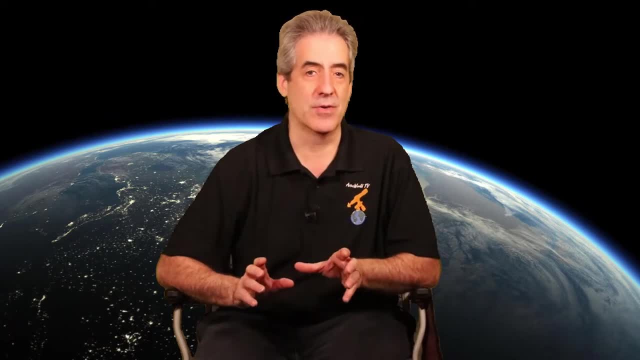 refractors need little to no adjustment of the optics. However, if you find that your refractor is out of collimation, then you need to adjust the optics. If you find that your refractor is out of collimation, then you need to adjust the optics. However, if you find that your refractor is out of 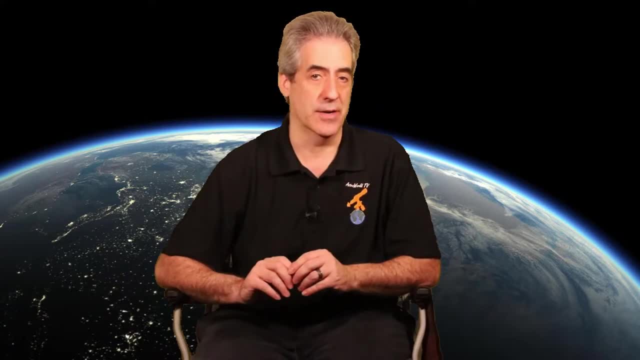 collimation, then you need to adjust the optics. If you find that your refractor is out of collimation, then you need to adjust the optics. If you find that your refractor is out of collimation, then you need to adjust the optics. Most distributors will fix it if necessary. 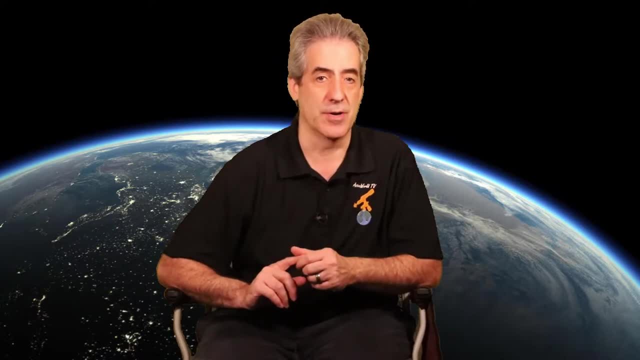 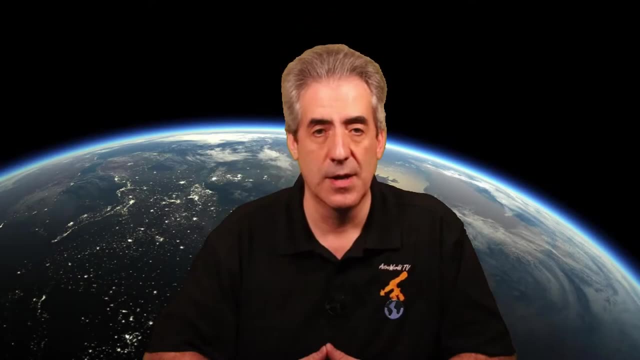 But still be safe and see your warranty information for each distributor. However, I have owned multiple refractors and none have had a collimation issue to this point. The second pro I want to talk about is a wider field. The refractor can give you a wider field, and that. 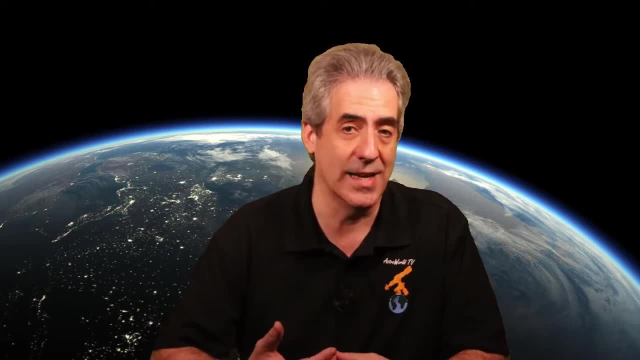 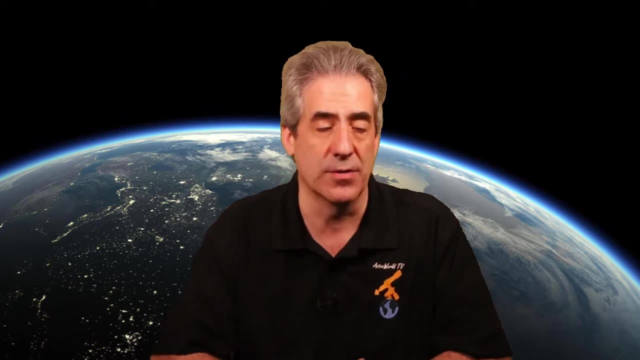 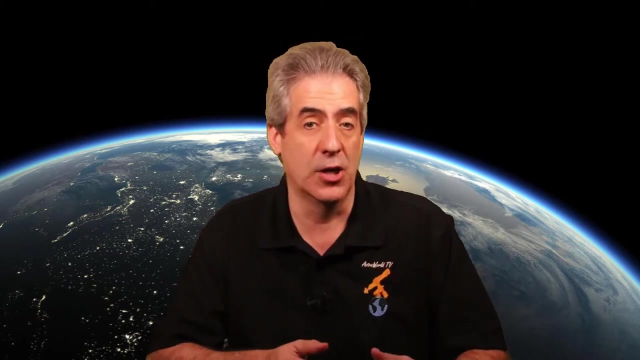 can make it a lot more forgiving as far as guiding is concerned. So it becomes a lot easier to guide because you're at that wider field. It will also allow you to fit larger deep sky objects on your chip because of the smaller focal length. So an 80 millimeter telescope at 400 millimeter focal. 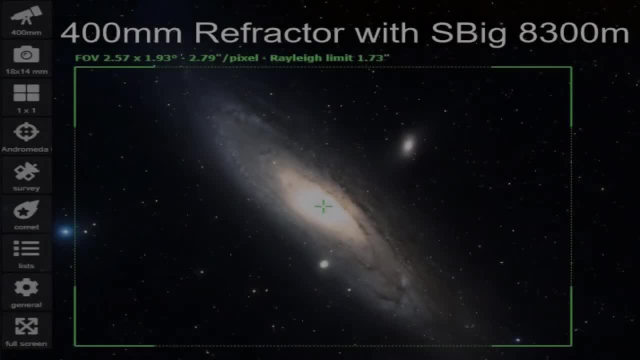 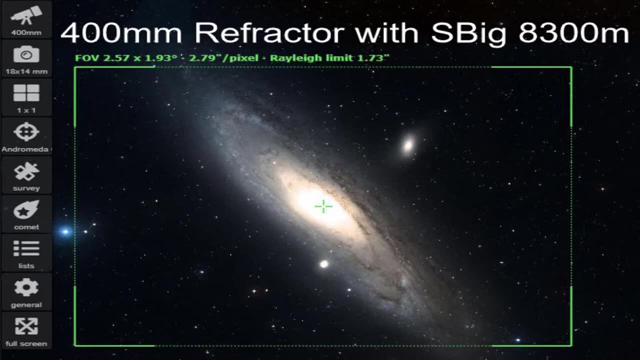 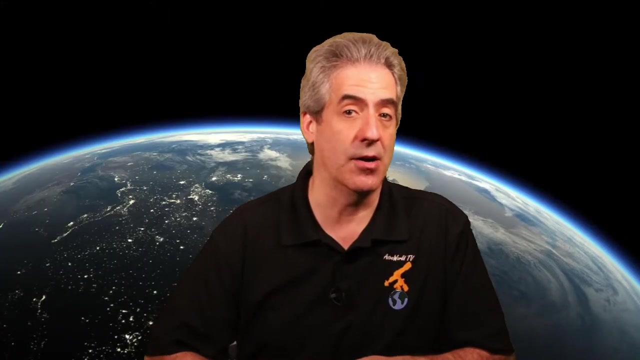 length will be able to fit natively the Andromeda Galaxy on the chip, depending on your chip size. However, the same in a Schmidt-Cassip grain without a reducer will probably just get the core of the Andromeda Galaxy. That's not to say that you can't fit the Andromeda Galaxy with a Schmidt-Cassip. 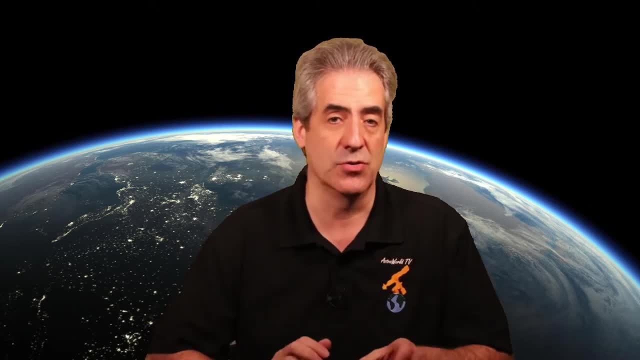 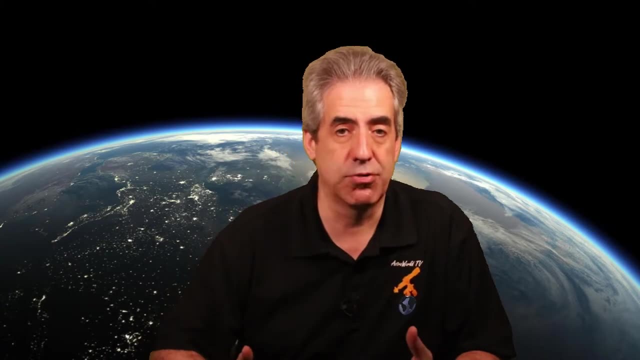 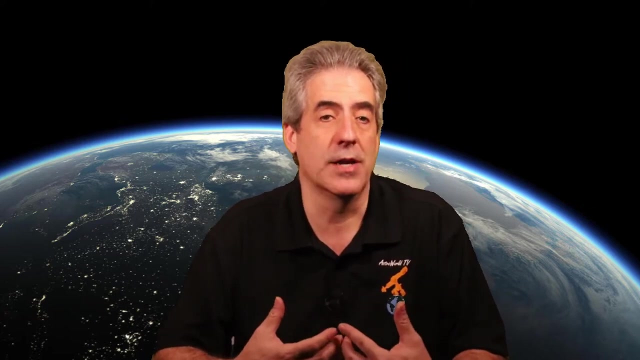 grain. You can, but you'll have to get a reducer and you'll have to do some post-processing in order to not see vignetting and that kind of stuff. The last pro that I'd like to talk about is image quality, And it may just be a personal preference for myself, but the image quality 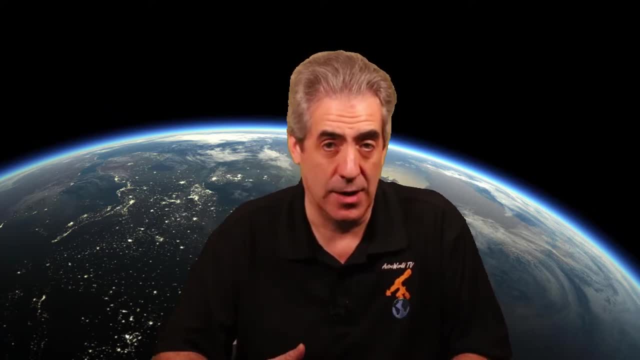 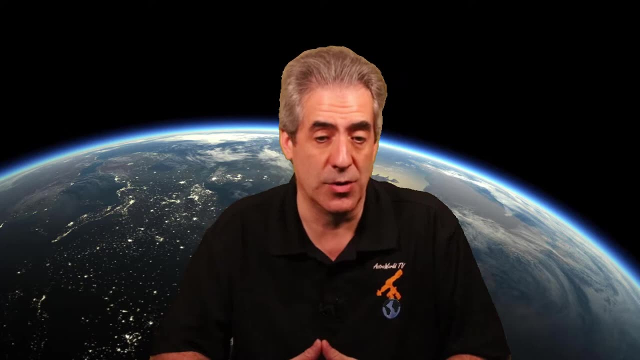 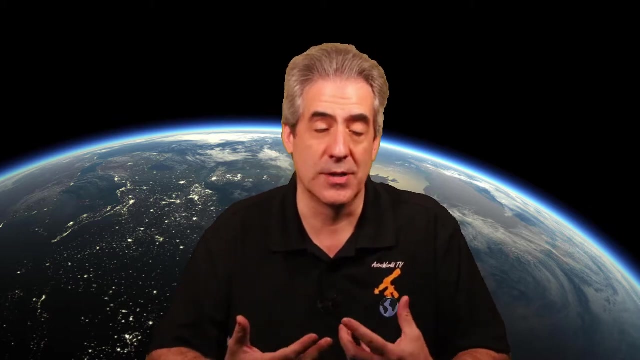 through a refractor can be outstanding, depending on your seeing, your transparency. all that kind of stuff gets compiled with your images. But stars, star colors. I find personally- and again, it's a Coke and Pepsi thing, but I think that the image quality in a refractor 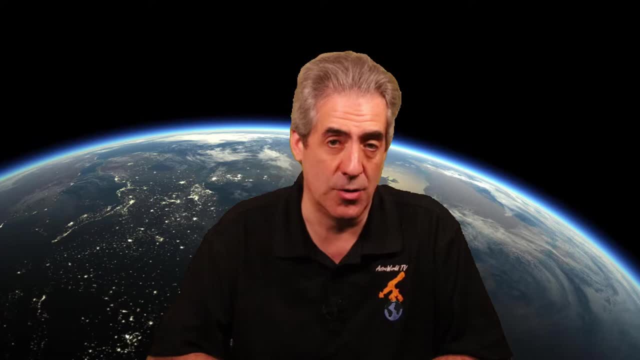 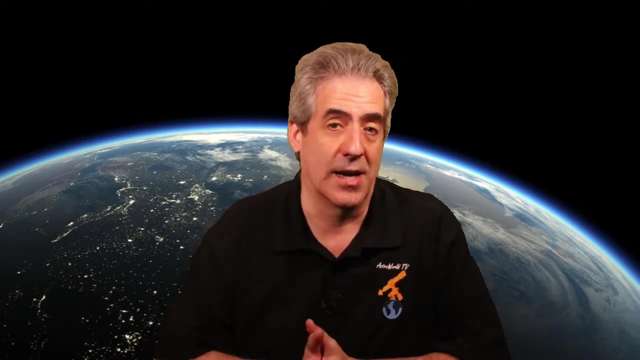 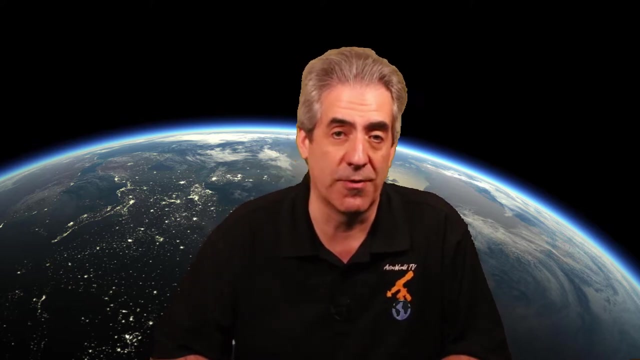 exceeds that of even Schmidt-Cassip grains and Newtonian reflectors. So image quality is bar none in a refractor as far as I'm concerned, And like I said, that is a personal preference. Out there that do image with different scopes that aren't refractors, can get similar results. 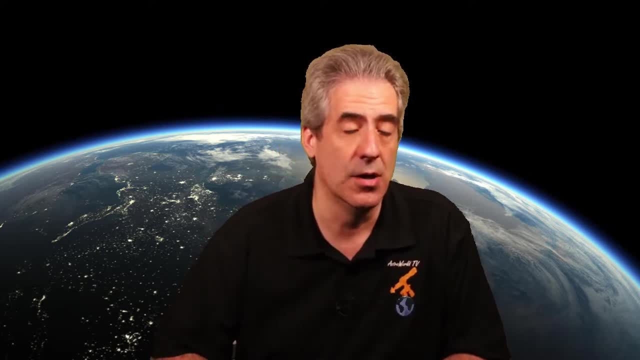 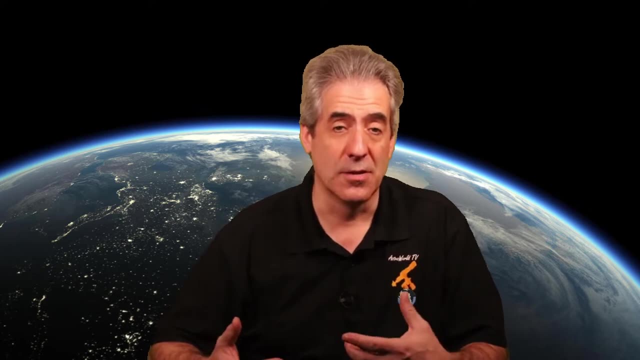 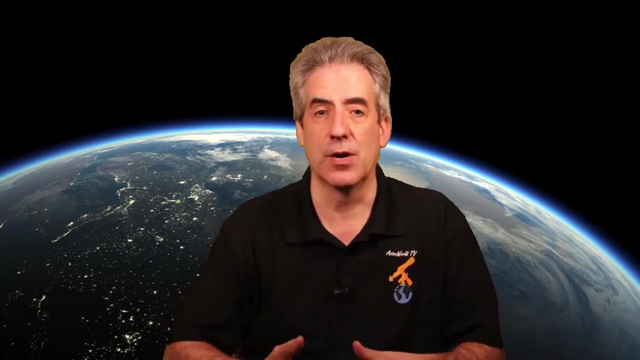 but I've found that I could get the results a lot easier with a refractor. And now the cons. The first thing that I could think about is that they're more expensive Because refractors are made of glass lenses. they tend to be more expensive per inch than their reflector counterparts. So, for example, you could buy an 8-inch Schmidt-Cassip grain or SCT for $1,200, where an 8-inch refractor will probably cost you about $20,000, plus you'll need a flatbed. 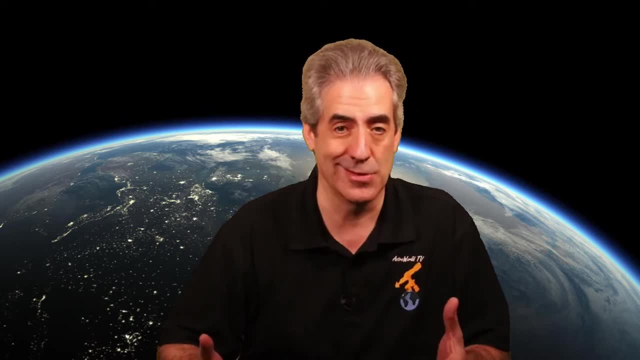 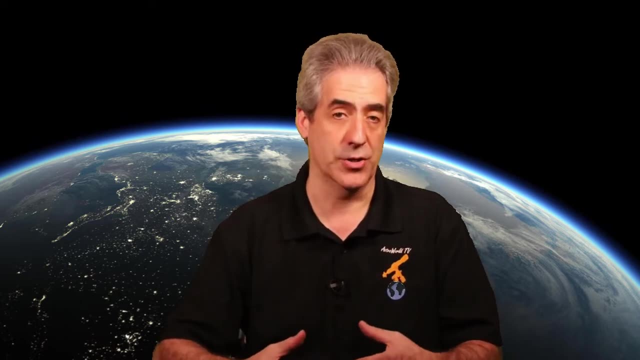 because the telescope is going to be about 7 feet long and weigh about 80 pounds. So the second con I could think about with refractors is that it suffers from something called curvature. Now, because a refractor is made with convex lenses, things at the center could be. 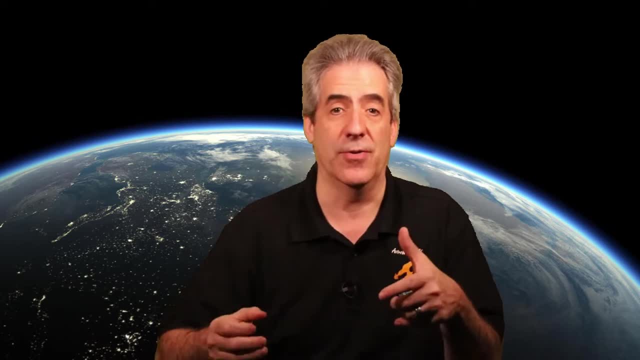 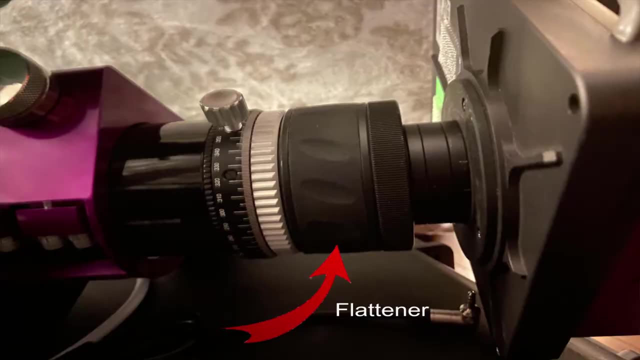 at focus, while the stars at the edges can be out of focus. Certain telescopes, like the Skywatch or SPREE, comes with refractors that are made of glass lenses. So if you're looking at a refractor- what is called a flattener- This will compensate for the curvature lens and make your stars in focus. 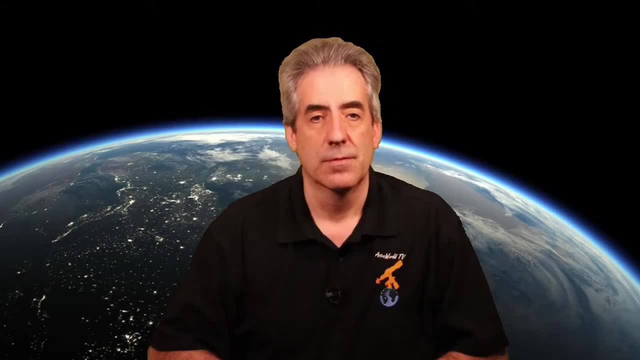 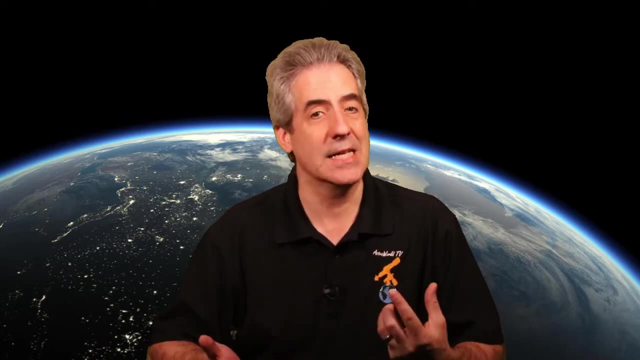 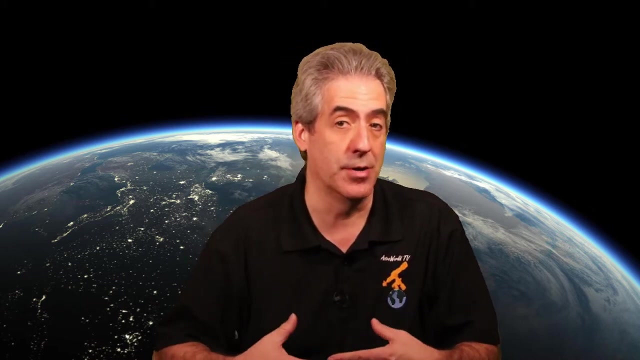 even at the edges. So the last thing on the con list is also on the pro list: the wide field. The wide field is great, but it's not suited for planetary or smaller galaxies and nebula. You'll need a longer focal length in order to get planetary or small nebula like the ring nebula. 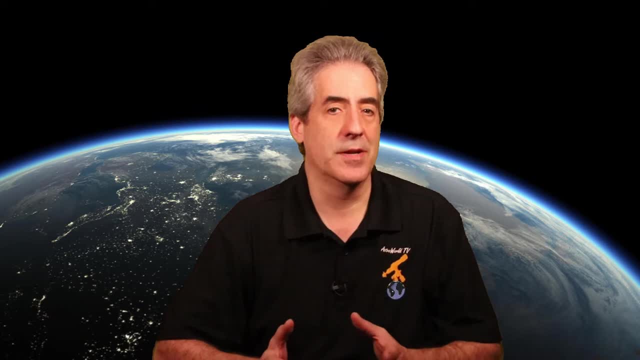 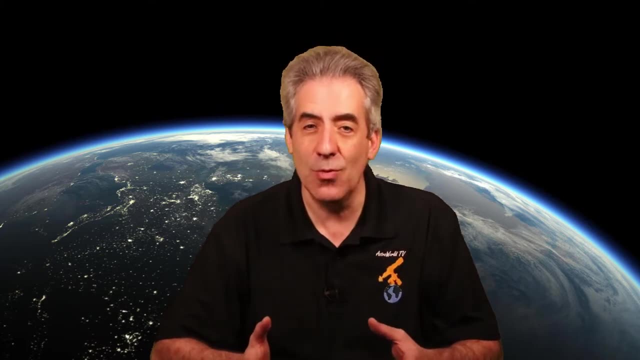 The refracting telescope is the oldest model of the telescope and has gone through a lot of upgrades in the past 400 years. However, it all comes down to what you want to image. Do you need a wide field of view with low magnification to get the Andromeda? 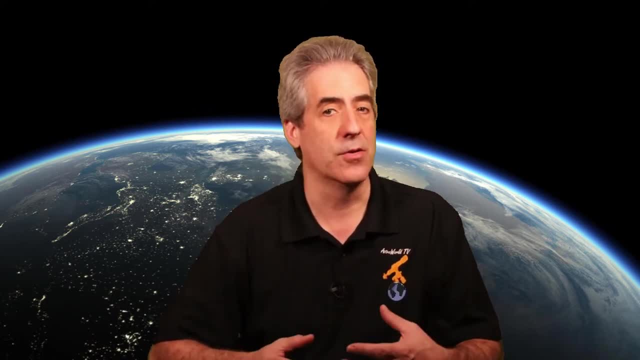 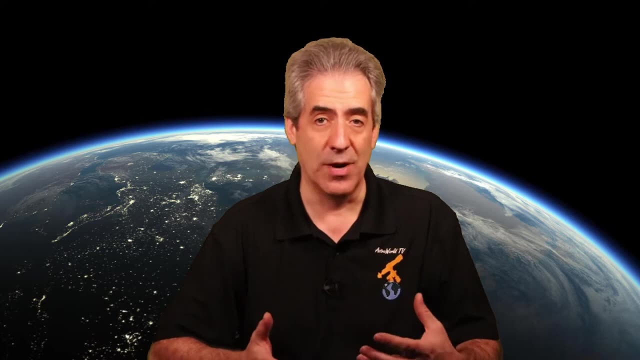 galaxy in one shot, Or do you need a long focal length in order to get into planetary astrophotography? Now, this is not to say that you can't get a long focal length. shorter you can. However, you need to add a focal reducer, which we will talk about in an upcoming video.